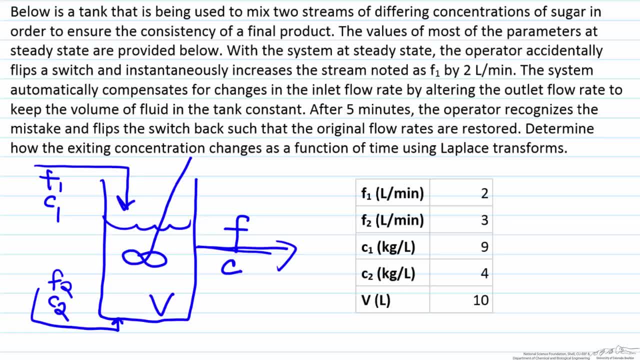 a tank of two streams with different concentrations of sugar being mixed together to get a desired final concentration. Note the fact that when the system is at steady state, we have the values that are provided on the right. We note the fact that we have a step increase. 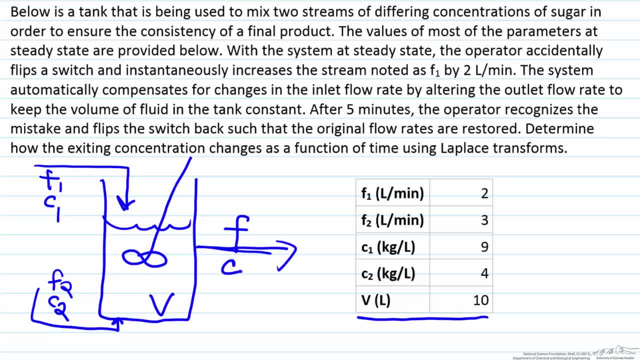 in F1 based on an operator error, but fortunately, the fact that in this problem we see that we have a step change, which happens in F1 by two liters per minute. However, this only lasts for five minutes and then the system is restored back to its original steady state. 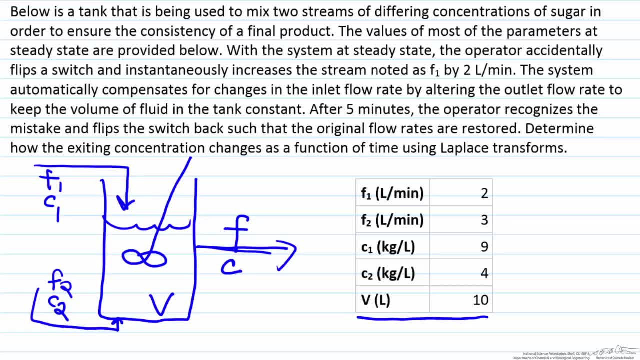 So the question is asking to determine how the exiting concentration changes a number of times per minute. So the question is asking to determine how the exiting concentration changes as a function of time, using Laplace transforms. So to start with, we'll develop a mathematical model for this process. An important point to note here is the fact that 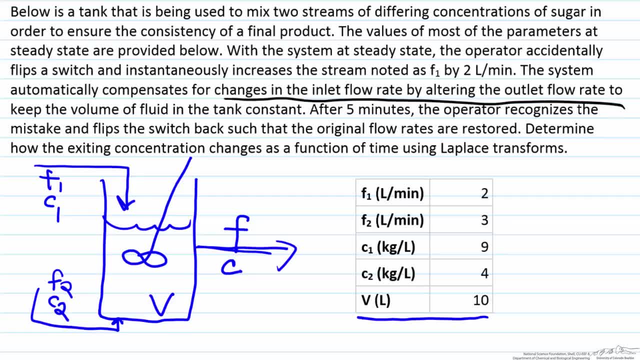 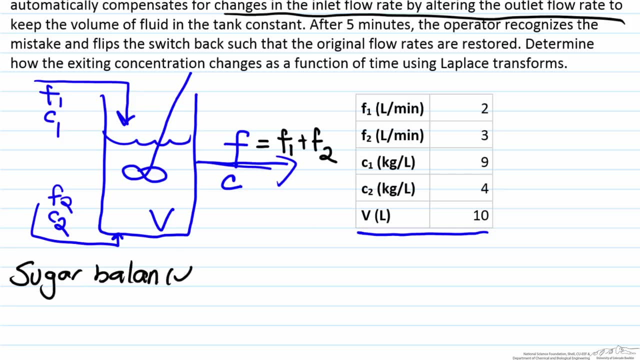 changes in the inlet flow rate are automatically compensated by altering the outlet flow rate. So in other words, a total mass balance is conserved. So in other words, F will always equal F1 plus F2.. But if we were to do a sugar balance here, what we would find is that the 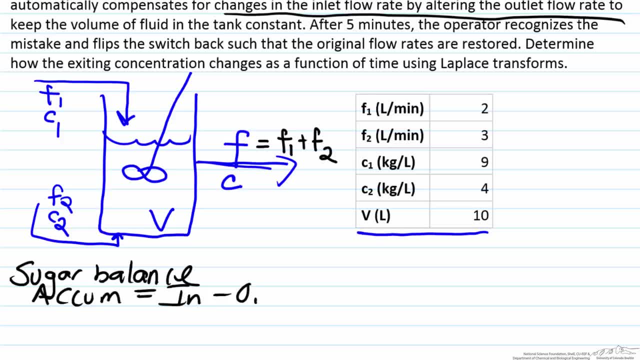 accumulation of sugar equals N minus F2.. This was an area of friction, which once again means that we're measuring the flow rate at different speeds. Now, the reason we're measuring the flow rate at different speeds is because, if we were to take an example of the product, which is the F1 that we just used, 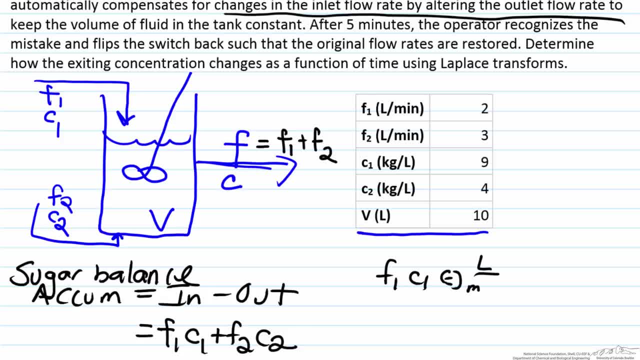 as an example of the flow rate that we just used in this video. we would be measuring the flow rate at different speeds, So we want to be able to see how fast this process will take. We have to make sure that the flow rate we're measuring is going to be in tune with 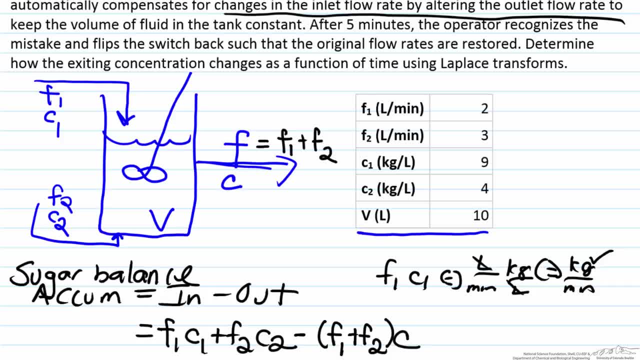 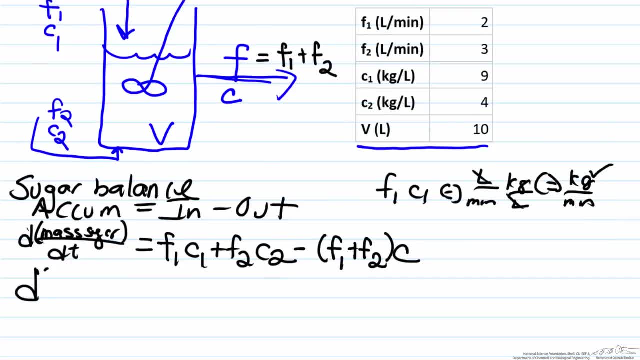 plus F2, multiplied by our concentration C, The accumulation will be derivative of the mass of sugar present. as a function of time, That will simply just be our volume multiplied by some sort of density, which in this case can be represented by concentration. So we 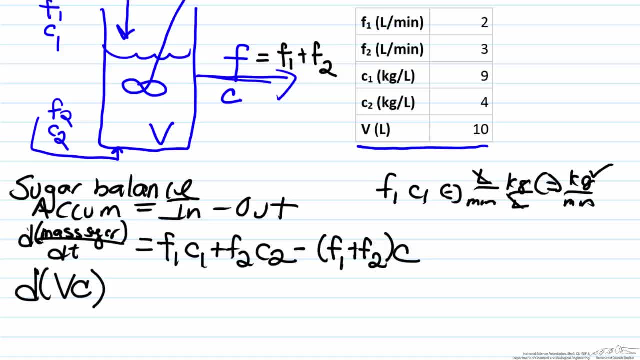 can multiply V. Here we're going to multiply times C because, since the tank is well mixed, the concentration exiting the tank is the same as the concentration inside the tank. So we have DVC, DT, We can factor the V out. So now we want to do, for simplicity's sake, 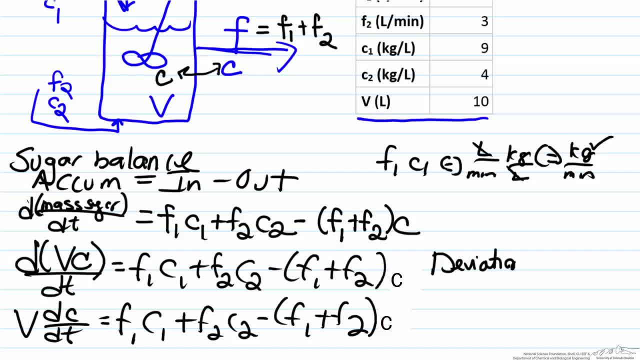 is: put this into deviation variables as we put this into Laplace transform. This is not a necessary step, but it makes some of our solution process a little easier. So here the things that can vary are C and F1.. Note, if we were doing this in terms of F, that would 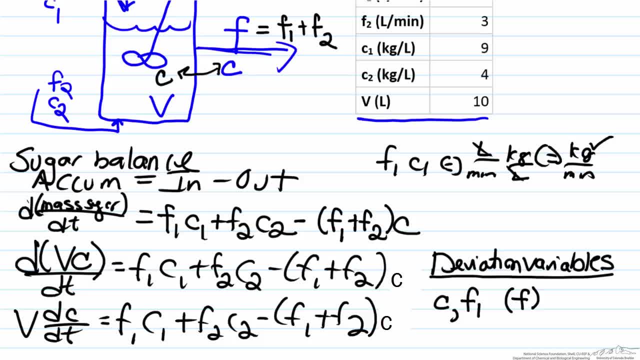 also vary, but in this case we explicitly wrote F as F1 plus F2 to make it a little easier to solve. So our deviation variables would be C prime and F1 prime. Remember the generic definition for a deviation variable is just the variable at a given time, minus. 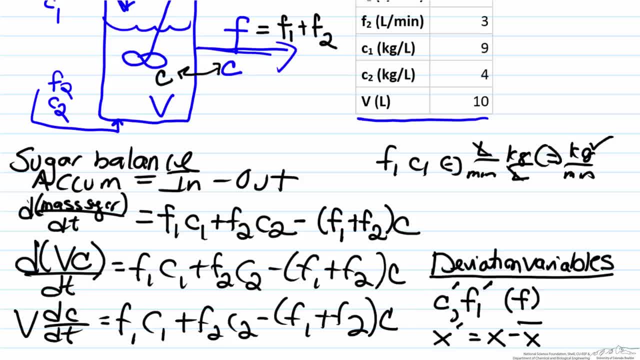 the steady state value. As we look at our final equation and we attempt to get it into Laplace domain, although everything is first order, an important point to note here is the fact that F1 and C are both variables, So we multiply them together. that is no longer. 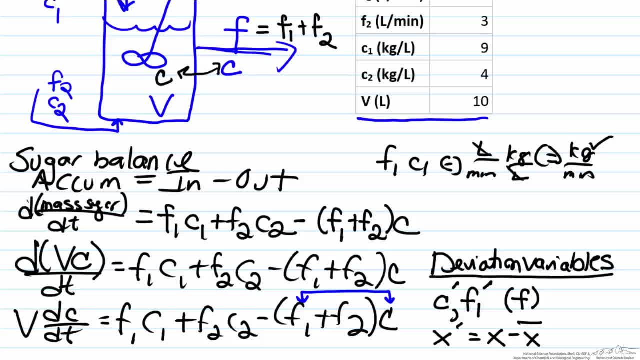 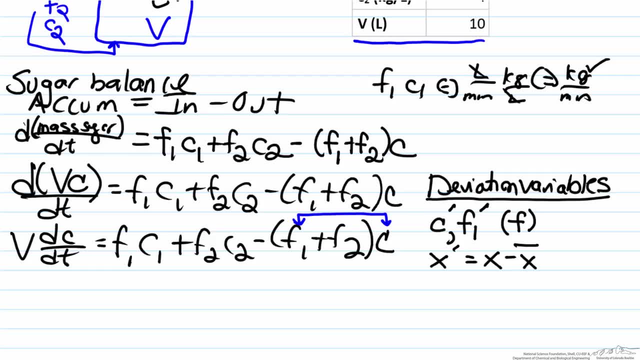 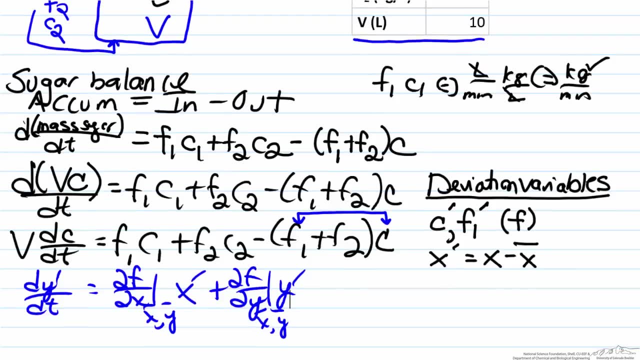 a linear term And there is no Laplace transform. So therefore that requires an overall linearization. Here we will use the equation to handle a differential equation that needs to be linearized, which is provided below. So here our two variables are C prime and F1 prime, So the left hand side will just be V times, DC prime, DT and 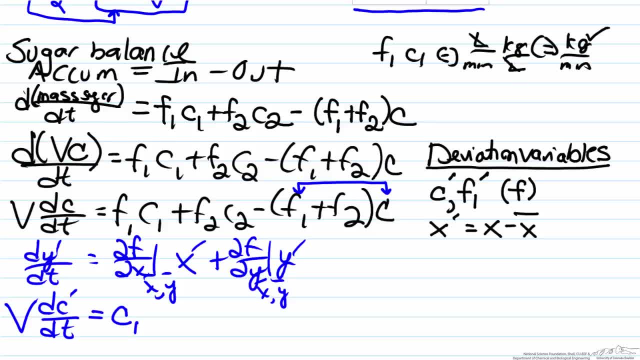 that will equal first our derivative with respect to F1, the second term goes to zero and the third term will be minus C. Let's put this in parenthesis because we are multiplying everything by F prime. But note, with C1 minus C, we have to evaluate it at the steady state value. so therefore C1 is. 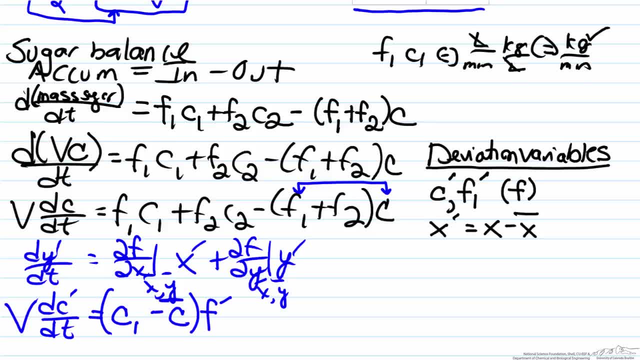 a constant, so there is no bar necessary, but C is not. So we are going to have to put a bar there, And for the C term we only have to look at the third term on the right hand side. so the derivative of that will be F1 plus F2 multiplied by C prime. Once again. 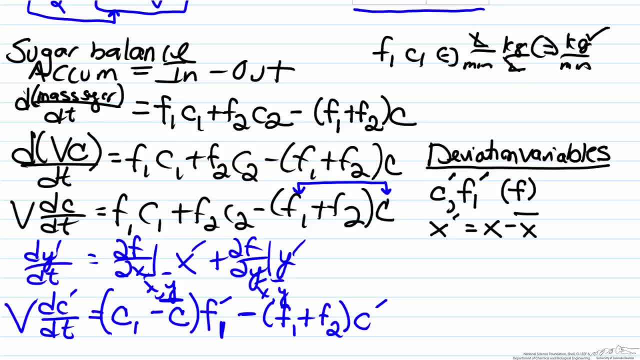 we evaluate at X bar, Y bar. in our case, the steady state is for C and F1. So we have to add a bar to F1. So F2 is a constant, so we don't have to concern ourselves with it. Now we take the Laplace. 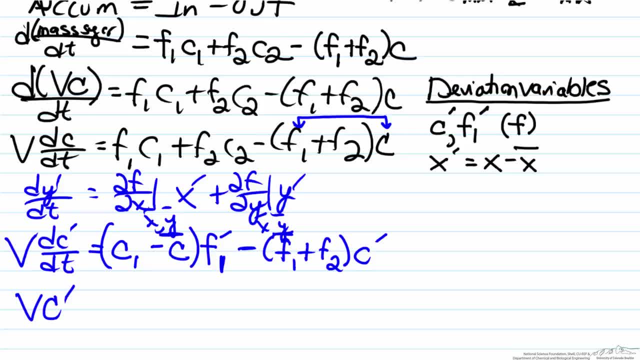 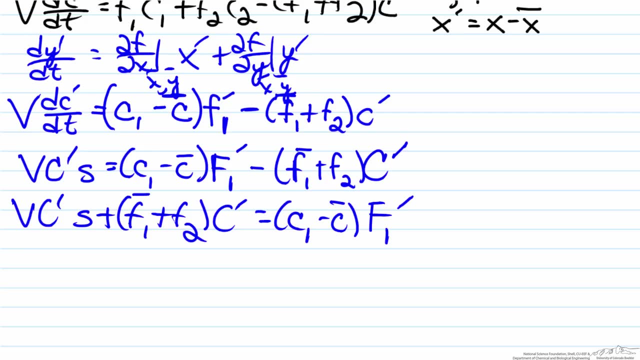 transform and we end up with V C prime. S equals C1 minus C bar multiplied by F1 prime minus F1 bar plus F2 multiplied by C prime. If we move the C prime it turns over to the left hand side and after a little bit more rearrangements we end up with our transfer function in standard. 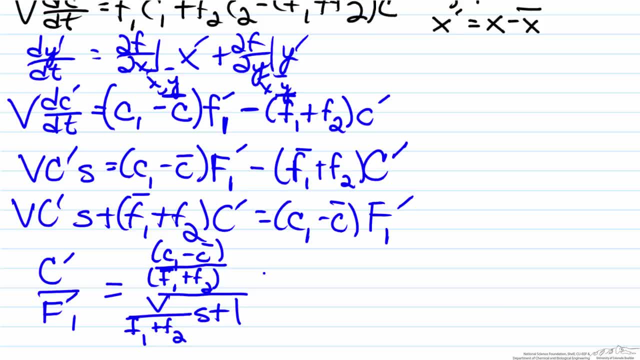 form. So we end up with a generic first order transfer. So we end up with a generic first order transfer. So this is our transfer function, where this term is our gain- which has units of concentration divided by flow rate. This is our value for the time constant, where 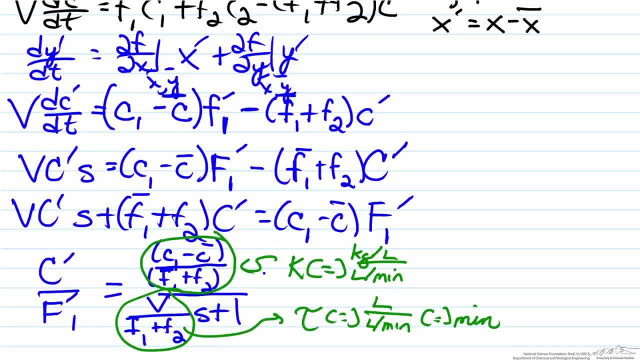 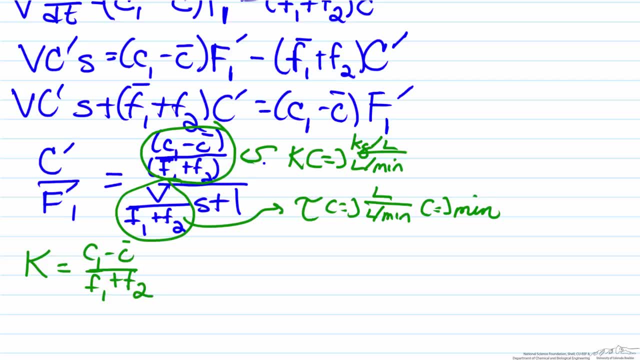 tau has units of minutes. Next we'll evaluate the value of the gain and the time constant. so we'll have to go back to the information we had at the beginning of the problem. So if we look at what we have at the top, we have the values for F1, F2, C1.. However, we 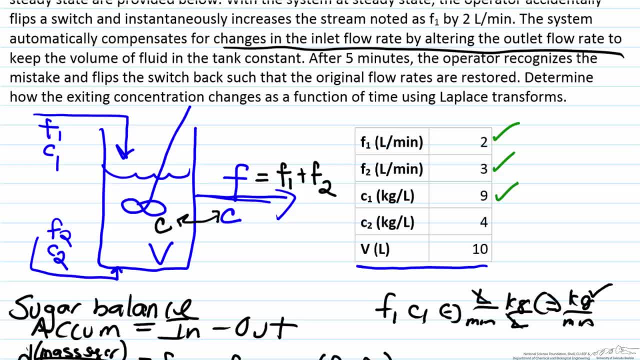 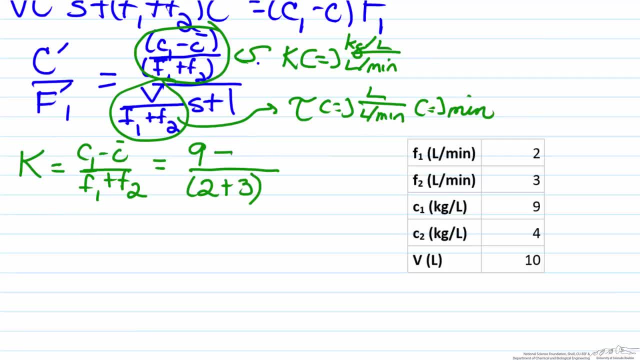 do not have the value for time, Which means that we are going to be adding up loss chúng for C bar. C bar can be obtained by using an entire mass balance at steady state. So to find C bar we'll use the same balance we had before, except the left hand side is. 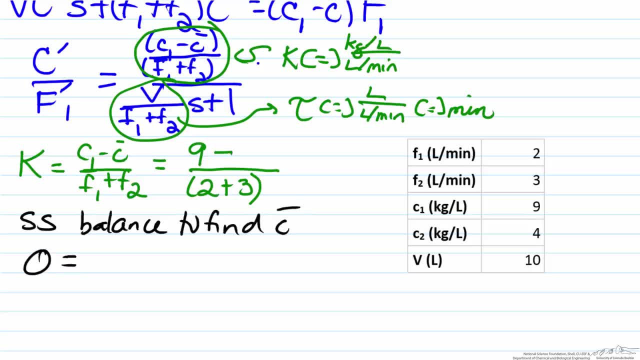 zero, And that will lead us with zero. equals F1C1 plus F2C2 minus F1 plus F2 multiplied by C. So in other words, C will equal F1C1 plus F2C2 divided by F1 plus F2, which equals: 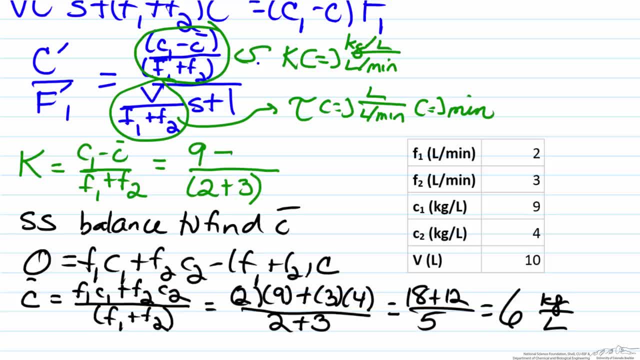 6 kilograms per liter, which is our value for C bar. So now we can solve for the gain as 3 over 5.. And then for tau we can solve for V over F1 bar plus F2, and that will just. 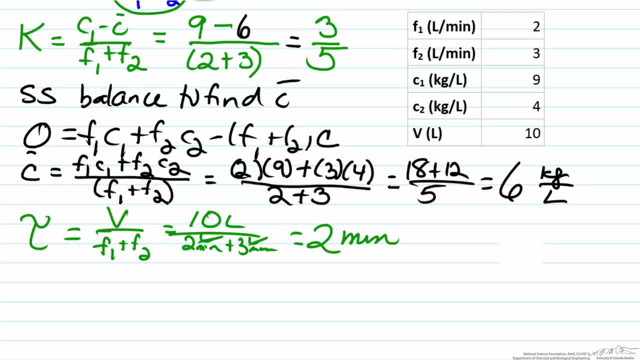 be 2.. So this means that our transfer function is: C over F1 prime equals three fifths divided by 2s plus 1.. But the next thing we have to do is we have to evaluate F1 prime in the Laplace domain. So to do this, we have to recall what was going on with our flow rate. 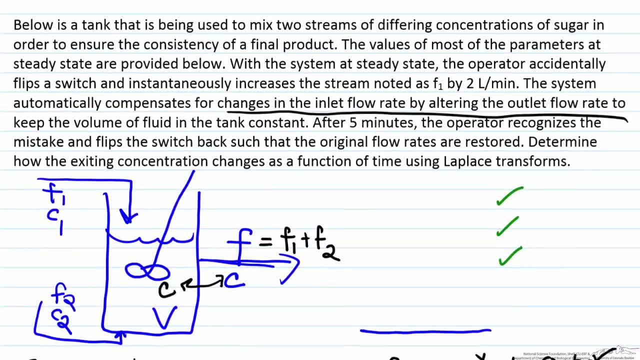 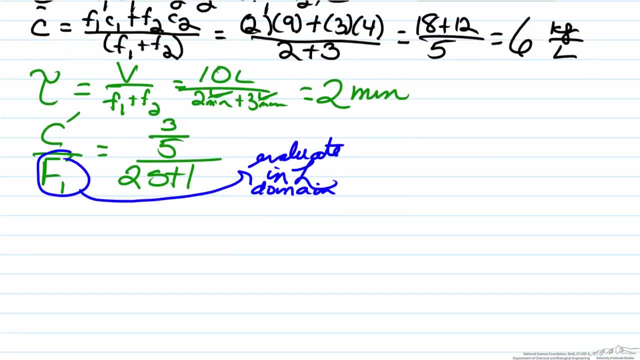 So what we see here is the fact that the operator flipped a switch and instantaneously increased the stream by 2 liters per minute, But then, after 5 minutes, the original flow rate was restored. So if we were to put this in mathematical form, what that would be saying is that F1. 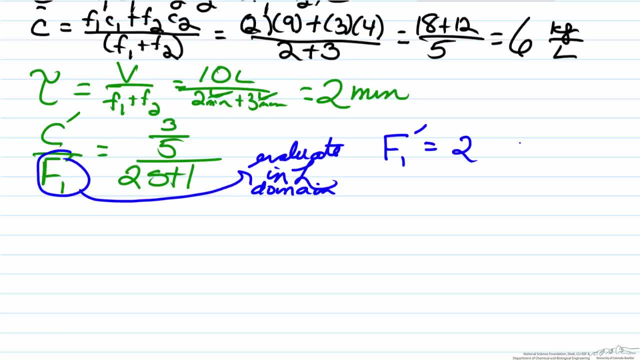 prime equals 2 for times between 0 and 5, and that F1 prime equals 0 for all else. for all other times, If this were to be graphed, it would represent what's known as a rectangular pulse, with the time axis from 0 to 5, and this being F1 prime going from 0 to 2.. So 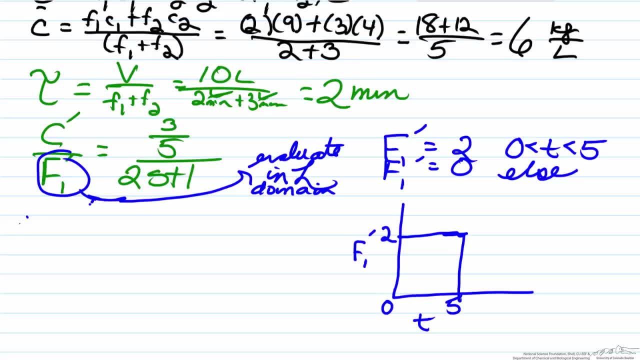 we'll use the definition of a Laplace transfer, Which is the Laplace of a function. So you have the integral from 0 to infinity of the function of the time domain, e to the negative st dt. So for our case here that will be: 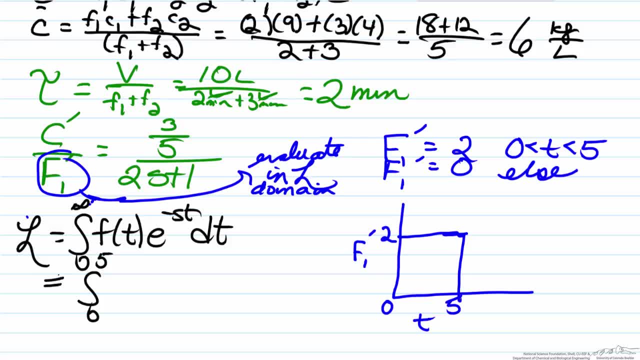 the integral from 0 to 5 of 2 e to the negative st dt, plus the integral from 5 to infinity of 0 e to the negative st dt. The second integral quickly goes to 0, and what we're left with? 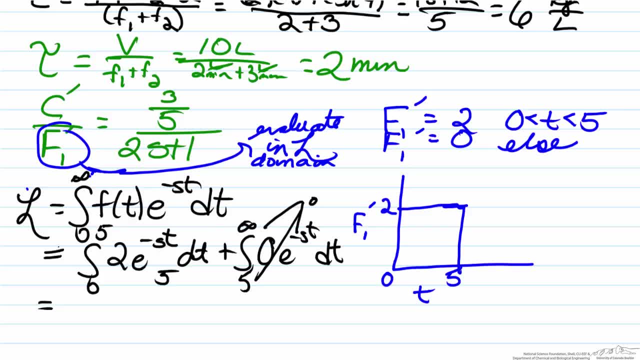 for our Laplace is: the integral will be negative: 2 over 5.. And so we'll have to say that this over s e to the negative st evaluated from 0 to 5.. You can rewrite this as 2 over s multiplied by 1. 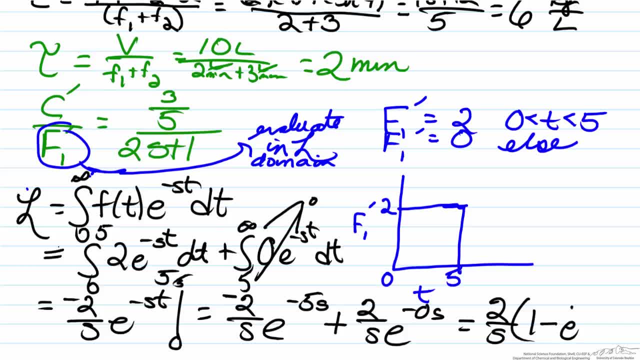 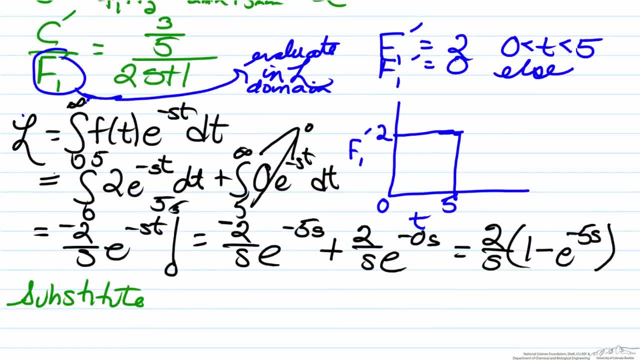 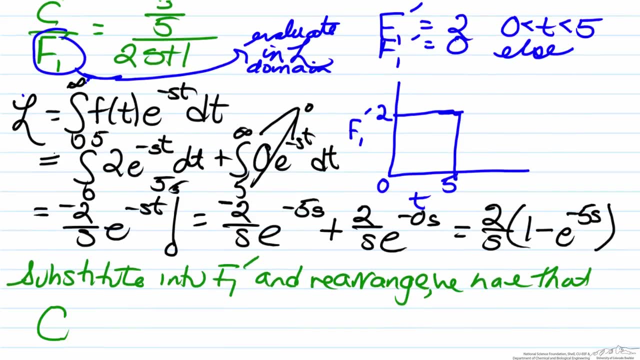 minus e to the negative 5s And this is what we'll substitute in for f1 prime. So when we substitute into f1 prime and rearrange we can restate the concentration c prime as 3 fifths over 2s plus 1. 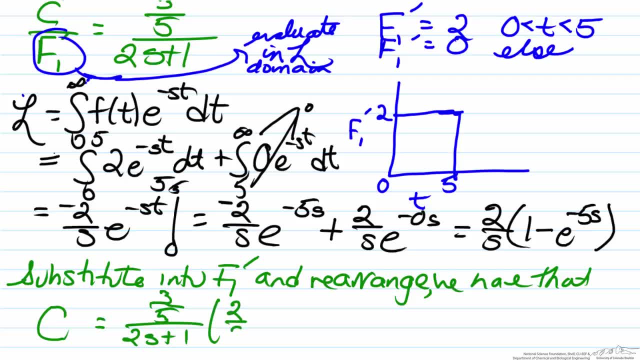 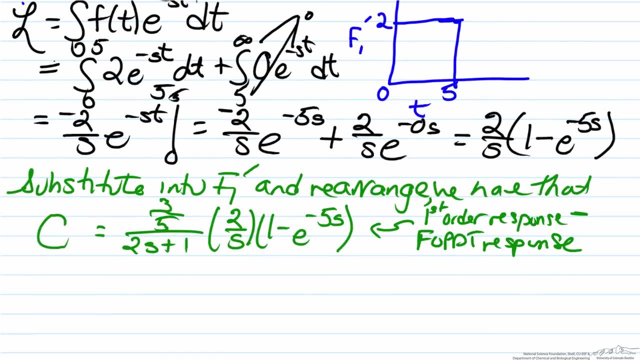 multiplied by 2 over s times 1 minus e, to the negative 5s. What this represents is a first order response minus a foftity response. So there are tables in which you can evaluate it explicitly. c prime, our deviation variable, will equal. So the first order response is of the form k: m times. 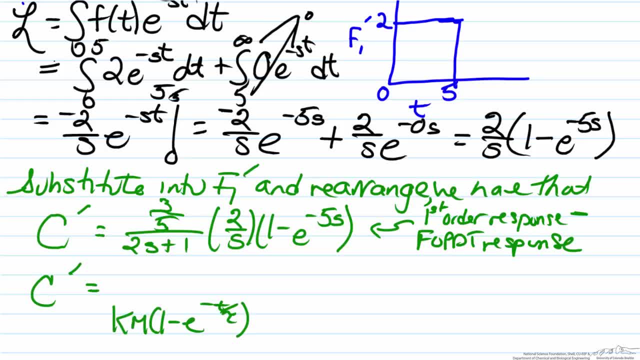 1 minus e to the negative t over tau. The foftity ability of the form k m multiplied by 1 minus e to the negative t over tau. But this t has to be replaced by the dead time, t minus t0..